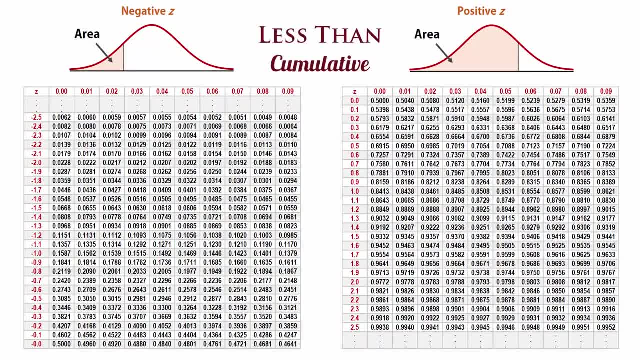 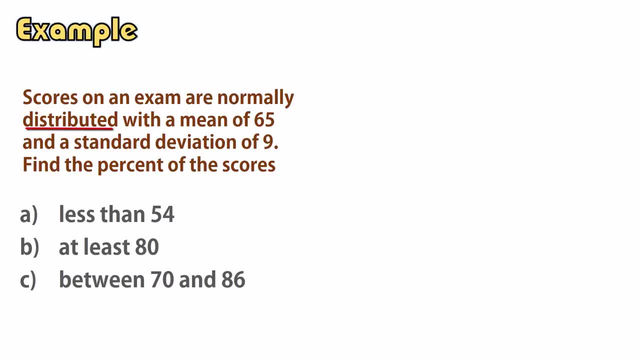 Standard, normal tables we will be using are the less than cumulative tables. They usually have the left tail of the distribution shaded and also have positive and negative parts. Let's look at an example. Scores on an exam are normally distributed with a mean of 65 and a standard deviation. 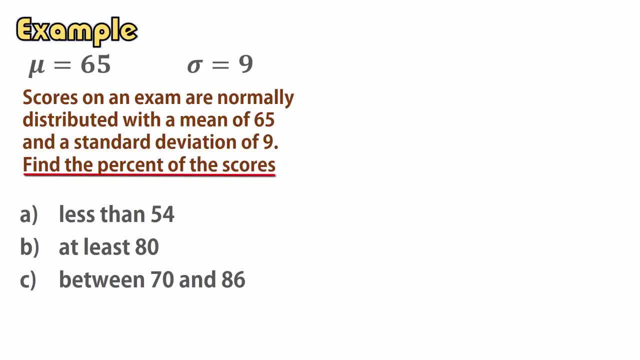 of 9.. We want to find the percent of scores satisfying A, B and C here. In A we want the probability that X is less than 54. So for X equals 54, the corresponding Z score is 54 minus 65 divided by 9, and that gives. 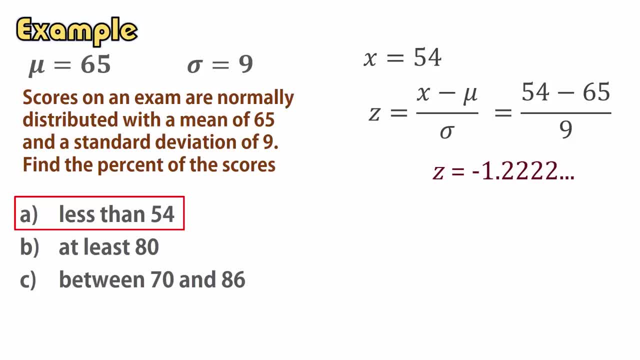 negative 1.2222. repeating: Since the Z table is set up to handle only two decimal places, we round this to negative 1.22.. We then go to the Z table and look up the area, For Z equals negative 1.22.. 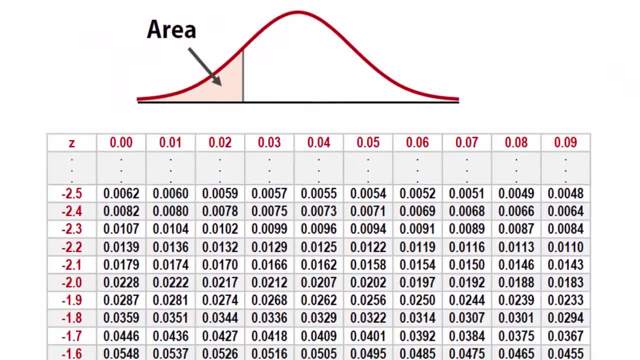 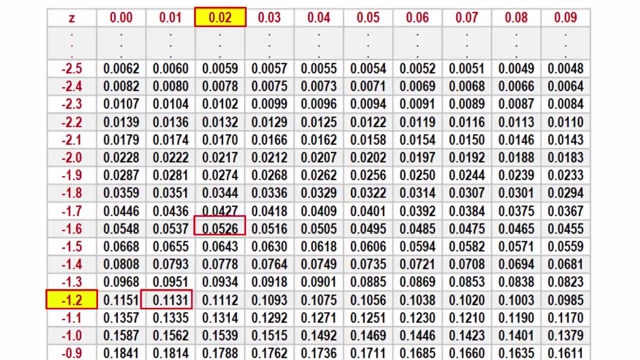 We go to the negative side of the table. Look for negative 1.2 in the first column and 0.02 at the top. The corresponding area here is 0.1112.. That is the area to the left. of Z equals negative 1.22 is 0.1112.. 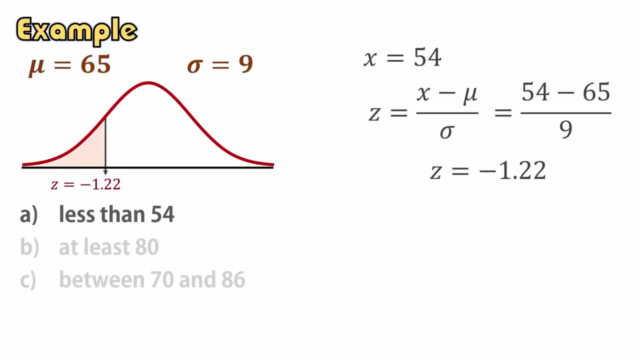 So, on this normal curve for Z equals negative 1.22.. The area on the left here is 0.1112.. The area on the left here is 0.1112.. Therefore, the probability that X is less than 54 is the probability that Z is less. 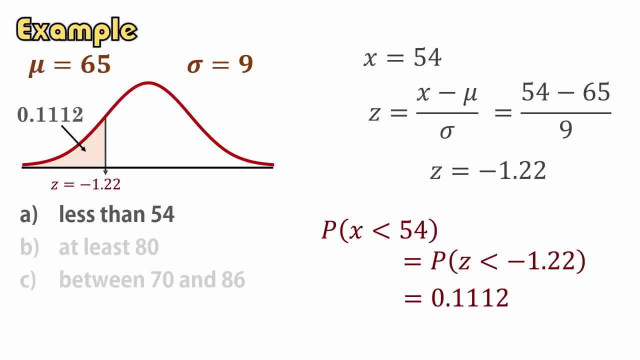 than negative 1.22, which gives 0.1112 or 11.12% In B, we want the probability that X is at least 80.. In continuous distributions, like the normal distribution, there is no distinction between X is at least 80 and X is less than 80.. 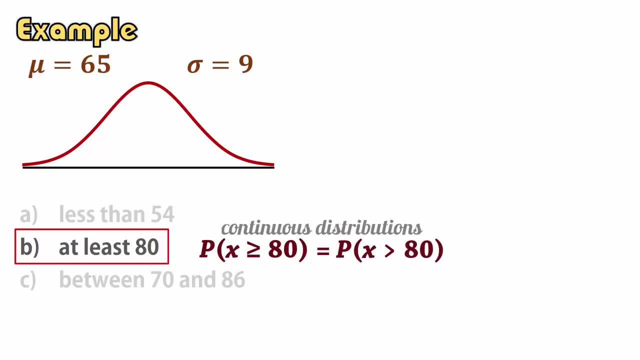 We apply the same approach in both cases. So for X equals 80, Z equals 80 minus 65 divided by 9, and that gives 1.67 to two decimal places. When we look that up in the Z table, by checking 1.6 under 0.07, we find 0.9525, which is the 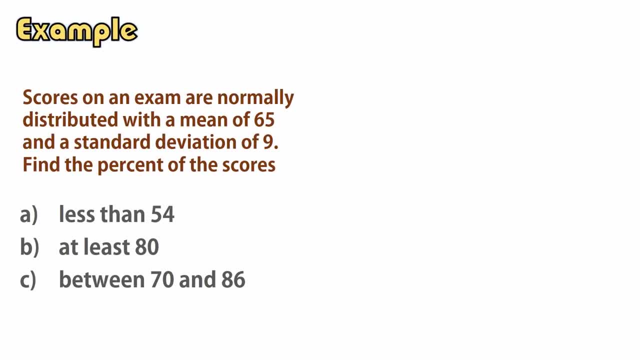 parts. Let's look at an example. Scores on an exam are normally distributed with a mean of 65 and a standard deviation of 9.. We want to find the percent of scores satisfying A, B and C here. In A we want the probability that X is less than 54.. 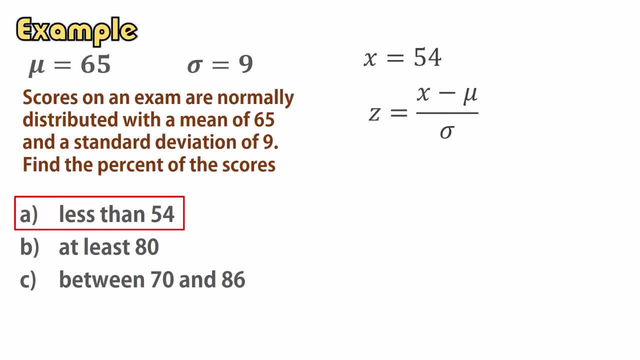 So for X equals 54, the corresponding Z-score is 54 minus 65 divided by 9, and that gives negative 1.2222. repeating. Since the Z-table is set up to handle only two decimal places, we round this to negative. 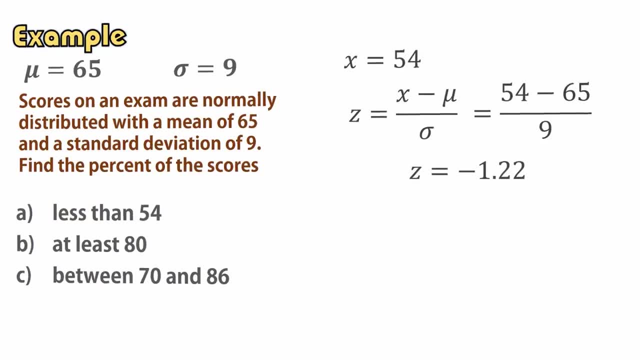 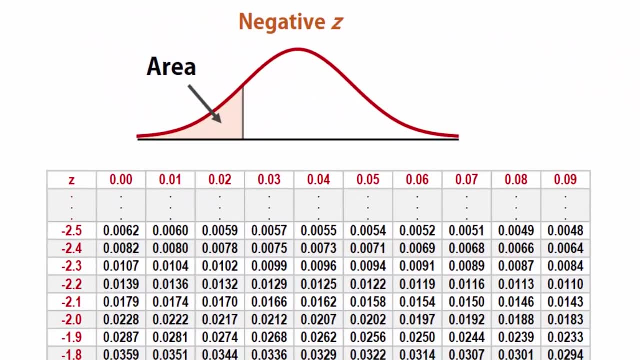 1.22.. We then go to the Z-table and look up the area, For Z equals negative 1.22.. We go to the negative side of the table. Look for negative 1.2 in the first column and 0.02 at the top. 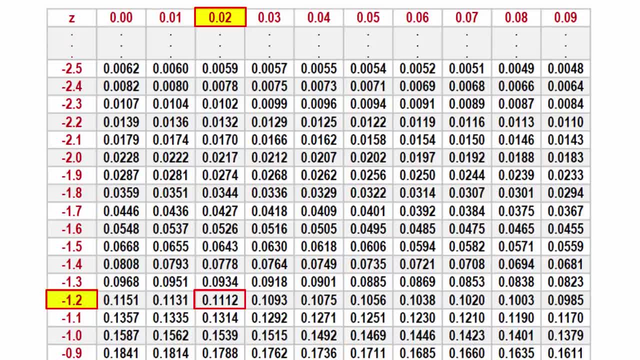 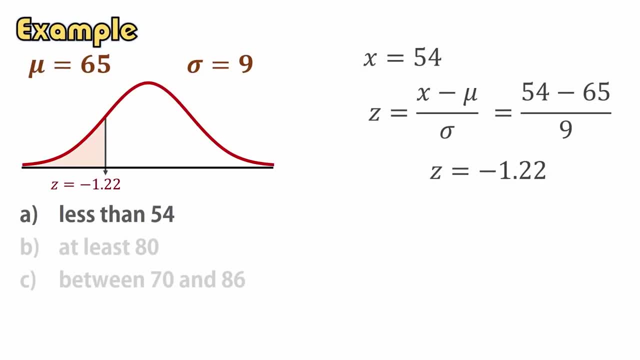 The corresponding area here is 0.1112.. That is, the area to the left of Z equals negative 1.22 is 0.1112.. So on this normal curve for Z equals negative 1.22,. the area on the left here is 0.1112.. 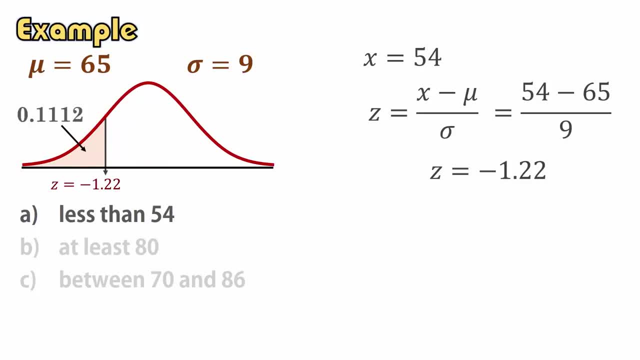 So, on this normal curve for Z equals negative 1.22,. the area on the left here is 0.1112.. Therefore, the probability that X is less than 54 is the probability that Z is less than negative 1.22,, which gives 0.1112 or 11.12%. 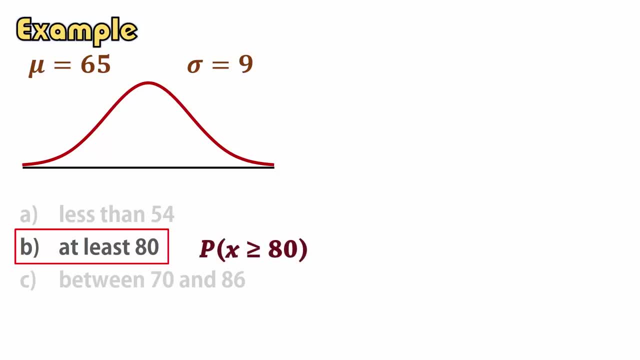 In B, we want the probability that X is at least 80.. In continuous distributions, like the normal distribution, there is no distinction between X is at least 80 and X is less than 80. Therefore, we want the probability that X is at least 80.. 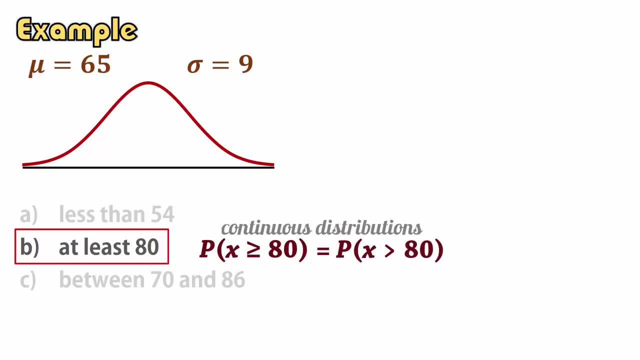 In both cases we apply the same approach. So for X equals 80, Z equals 80 minus 65 divided by 9, and that gives 1.67 to two decimal places. When we look that up in the Z table, by checking 1.6 under 0.07, we find 0.9525, which is the 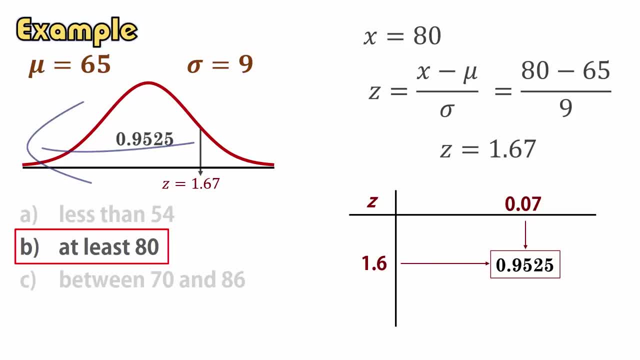 area to the left of Z here. We then subtract it from 1 to obtain the greater than 80.. However, we are now dealing with the given area. We now have the area to the left of Z. We then subtract it from 1 to obtain the greater than 80..